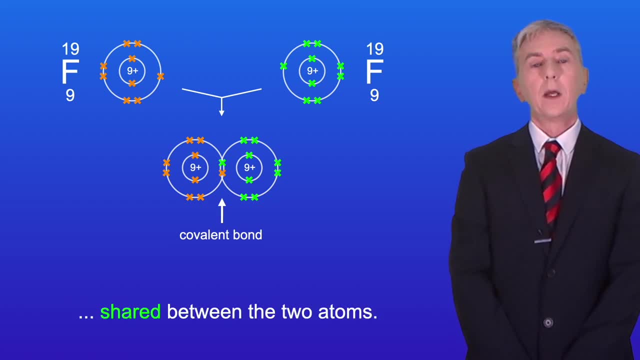 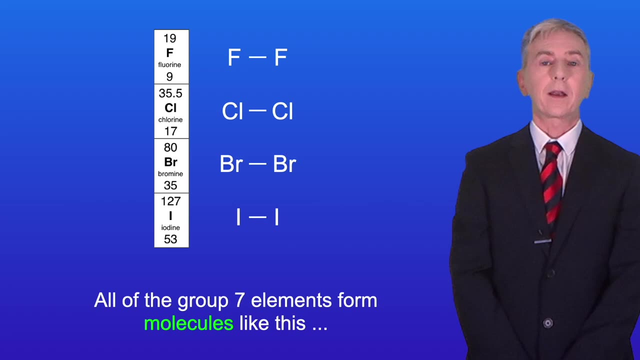 pair of electrons shared between the two atoms. We now call this the fluorine molecule, F2.. All of the Group 7 elements form molecules like this, with two atoms joined by a covalent bond. Now here's a key fact that you need to learn: Group 7 elements form covalent compounds when. they react with other non-metal elements. I'm showing you here a chlorine atom and a hydrogen atom, and remember that hydrogen is a non-metal. Both of these elements require an extra electron to achieve a full outer energy level and they do this by forming. 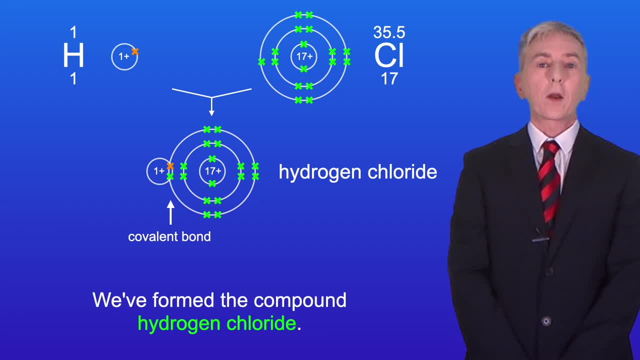 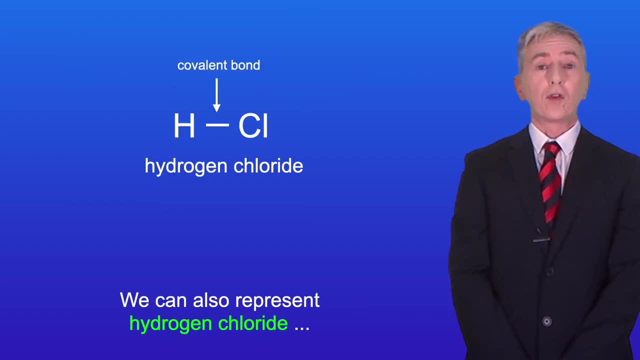 a covalent bond like this, We've formed the compound hydrogen chloride, and hydrogen chloride is a covalent compound. We can also represent hydrogen chloride by using a stick to show the covalent bond. All of the halogens form covalent compounds when they react with other. 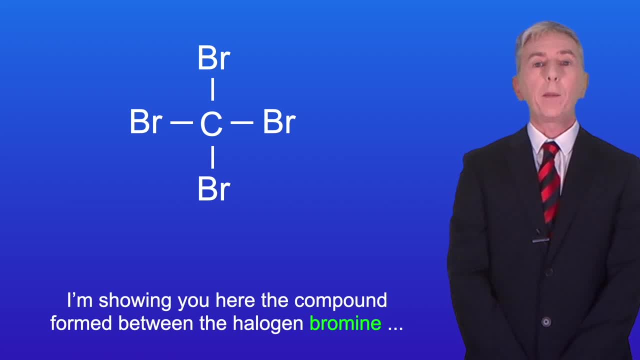 non-metal elements. I'm showing you here the compound formed between the halogen bromine and the non-metal carbon, and again we can see that this is a covalent compound. Here's a compound between the non-metal phosphorus and the halogen iodine, and once again you 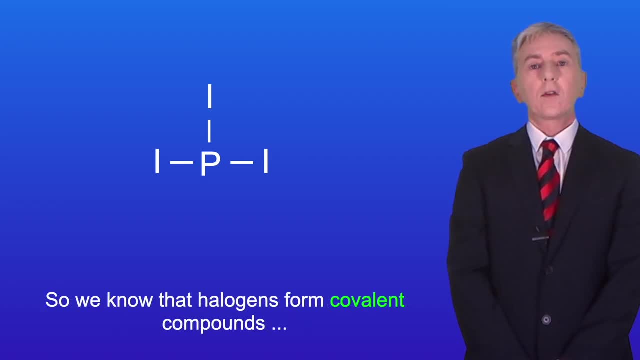 can see that this is a covalent compound. So we know that halogens form covalent compounds with other non-metals. But what happens when halogens react with metals? Here's another key fact that you need to learn: When halogens react with metals, they form. 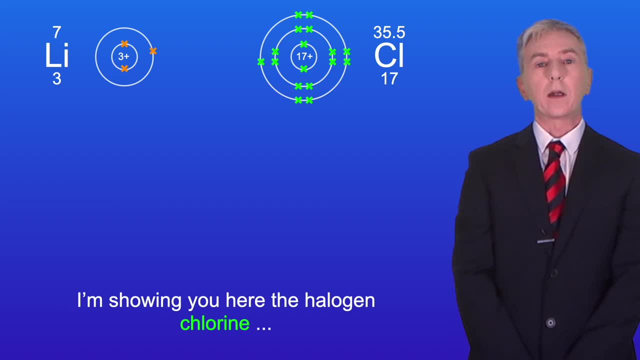 compounds. I'm showing you here the halogen chlorine reacting with the metal lithium. Lithium has one electron in its outer energy level and chlorine has seven electrons in its outer energy level, just like all the other halogens. A chlorine atom has 17 protons. 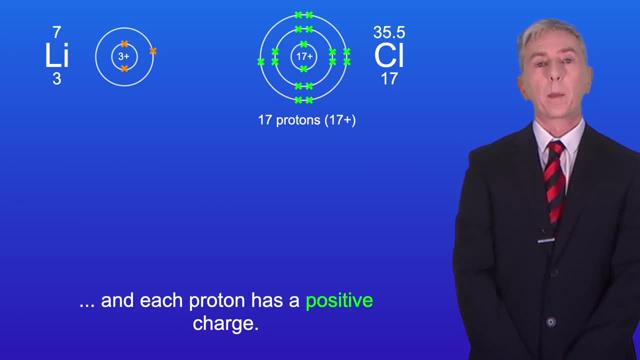 in its nucleus and each proton has a positive charge. Chlorine also has 17 electrons and each electron has a negative charge. So in a chlorine atom charges on the protons and electrons cancel and the chlorine atom has no overall charge. 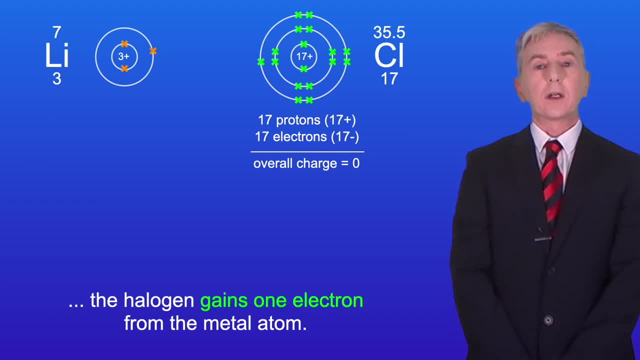 When a halogen atom reacts with a metal atom, the halogen gains one electron from the metal atom. So when chlorine reacts with lithium, the chlorine atom gains one electron from the lithium atom. like this, The chlorine atom still has 17 positive protons in its nucleus.